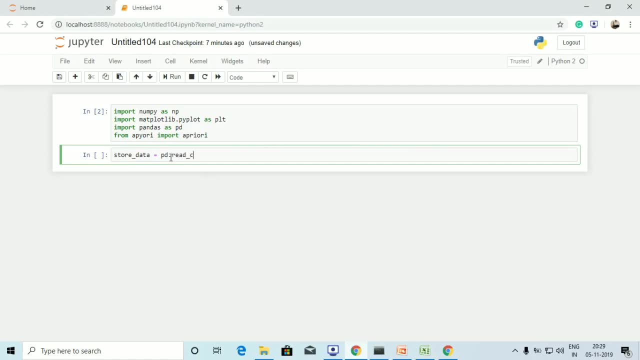 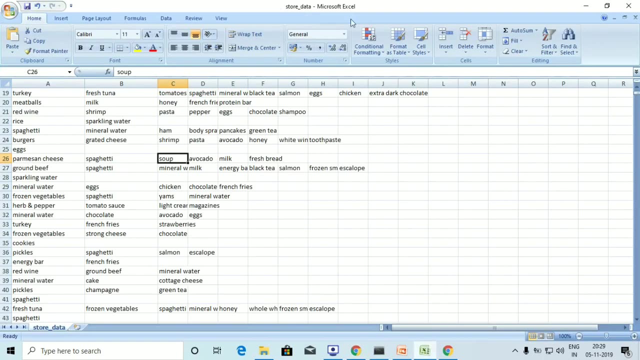 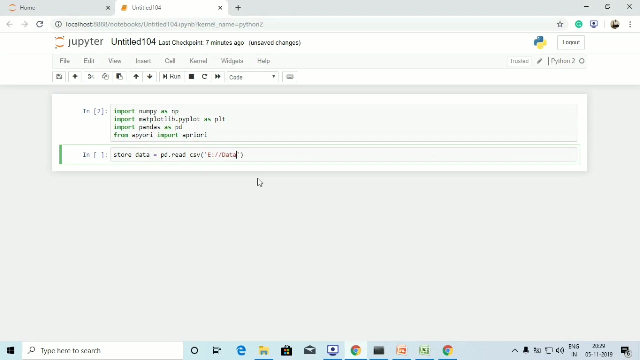 pd dot read underscore csv. and inside the packet we are going to provide this file, which is available in the location which is e, colon, double slash data sets. double slash the file name which is store underscore data dot csv, and we are going to make sure to keep the header as none, as we don't need the header. 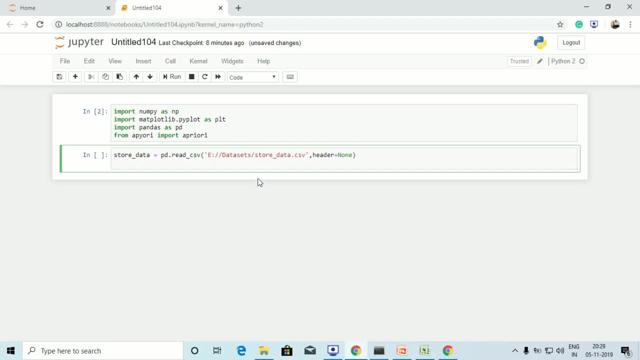 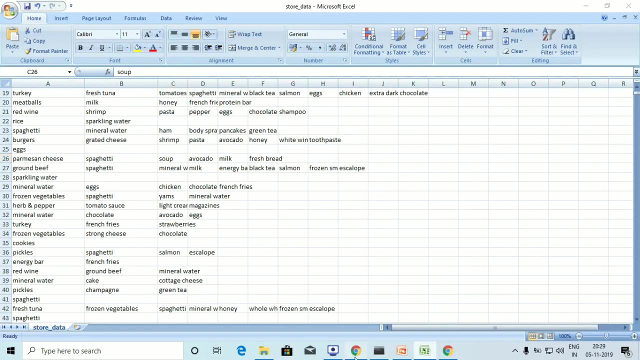 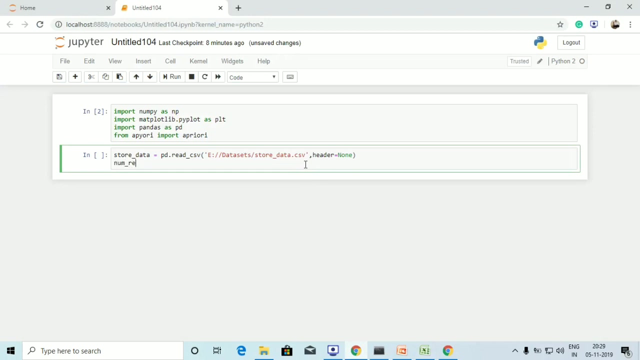 So first step is completed. So we have read the file, which is the data stored in csv, which is available in E colon. So now we read the data. Next step, let's see the note of the record, which is by creating a variable called num underscore records, And we are going to provide 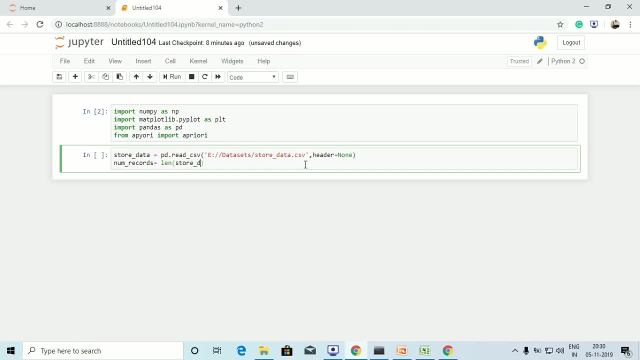 le n keyword along with store underscore data, which is this variable in which file location is there? So let's try to view the length of the store underscore data variable so that we could know the file size of the store underscore data. For that we are going to print number. 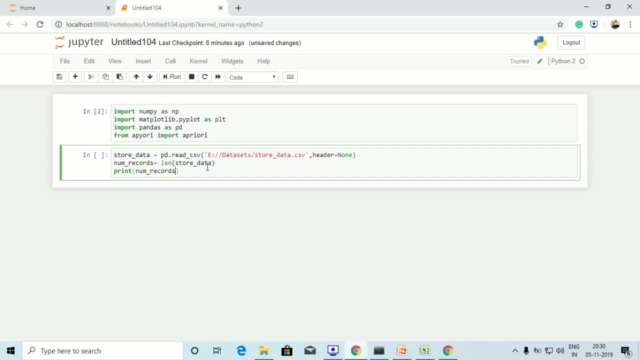 underscore records. By printing this, what will happen? it will come over here and it will calculate the length of store underscore data, which is this file. Let's now go ahead and print the program. Here we go. We have got the output as sign 501.. So the length of this file is sign 501. 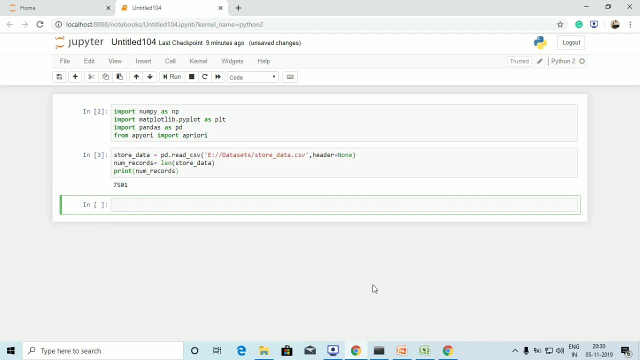 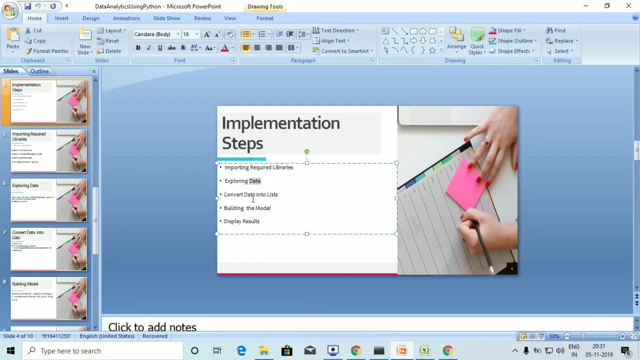 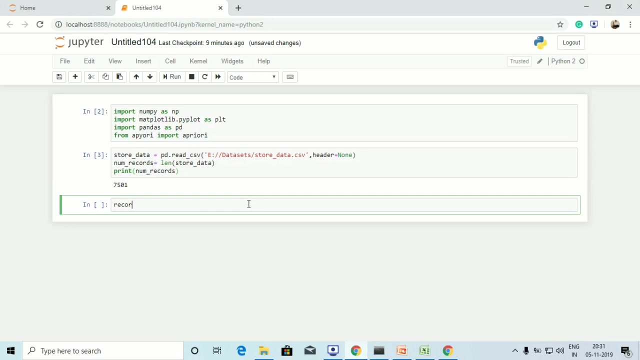 Now, as we have read the file, so we are exploring the data. Let's now build the model and also convert data into list. For doing that, first we are going to create a variable called records and keep this blank, as it is Now what we are going to do. 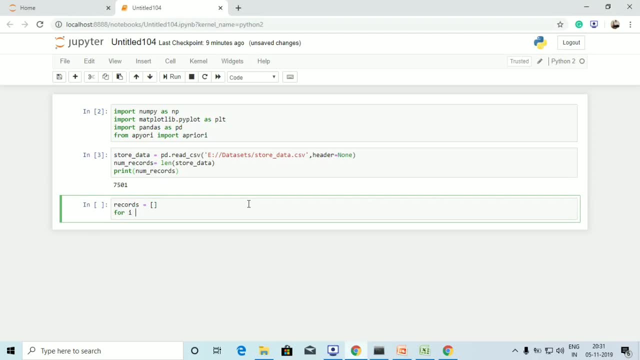 we are going to create a for loop by putting i in range and inside the brackets. we are going to start with the value zero and the second would be num underscore records, to make sure that we do not cross the length of the number records, which is seven five zero one. So so we have provided the value of zero. 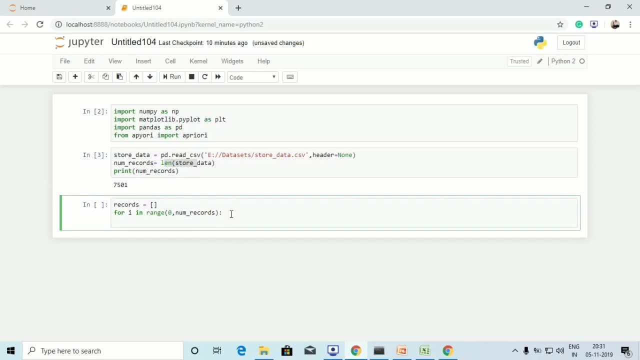 comma num underscore records. Let's go inside the for loop and use the append method, which is records dot append, and inside the bracket we are going to string and store dot, store underscore data, dot values into i comma, g, i, j, And also we are going to use one more. 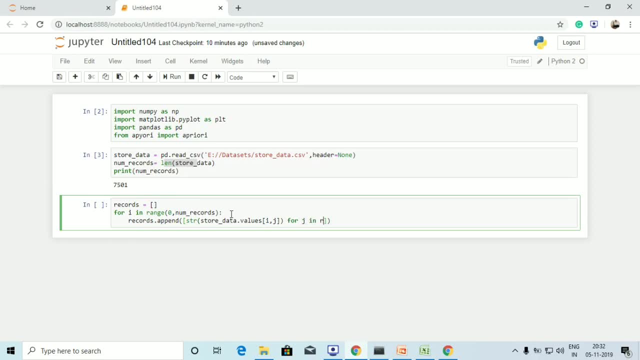 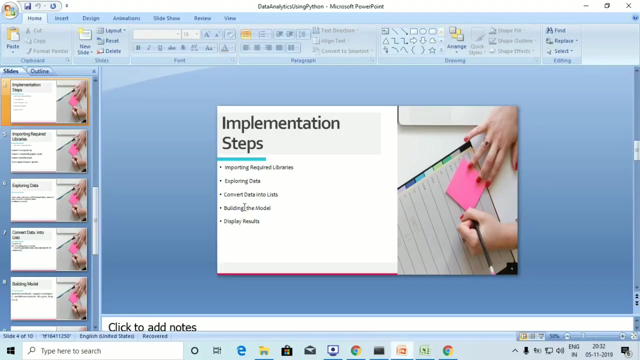 for loop, which is for j in range of zero, comma 20.. By using this code, we will be able to. So we are going to append the records and store the values for underscore data in IG. So this is how we do that. The next step is you're going to build the model which is going to provide these a priori. 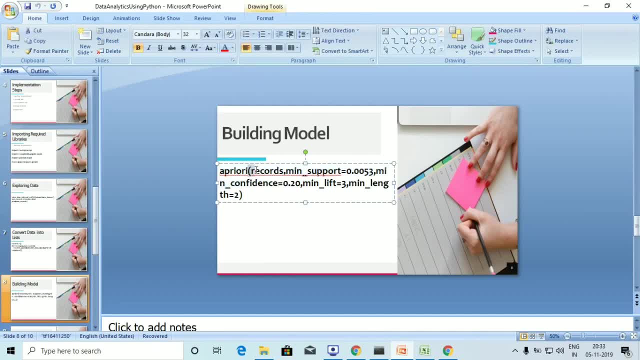 that is so for building the method and also will provide the other stuff, that such as support, confidence and lift, which we have discussed in the earlier tutorial. So we are going to provide a minimum value for support, confidence, as well as lift and length, to make sure that we get the data as we want. 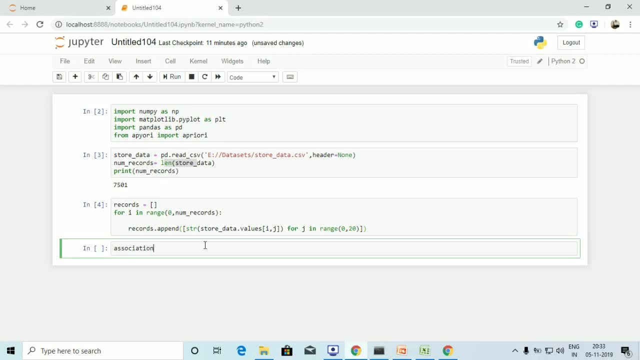 Let's go ahead and build the model, which is I'm going to provide association underscore rules as a variable. equals to a priori, a priori and inside that I'm going to for the records, followed by minimum underscore support as the value. I'm giving it a value. 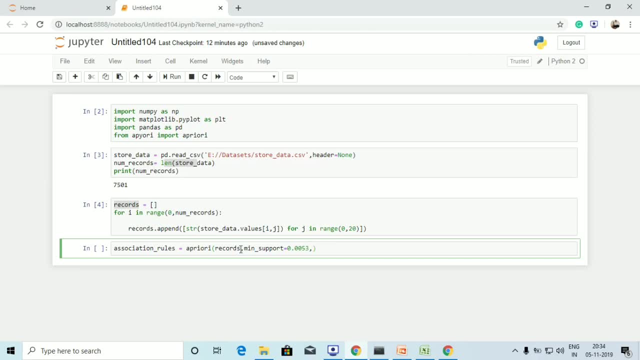 as 0.0053 as a minimum support value, followed by minimum underscore confidence, as I'm going to provide the value for it as 0.20, and for minimum underscore left, I'm going to provide the value as 3, and for minimum underscore length, Let's say we'll give it as 2.. So here, 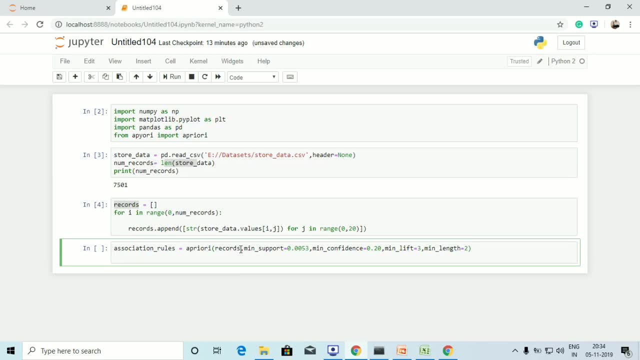 we go. We have built the model. Let's now put this into a list. For doing that, I need to create one more variable as association underscore results. So lah, Belarus equals to list of, and we didn't do this here. It is association. 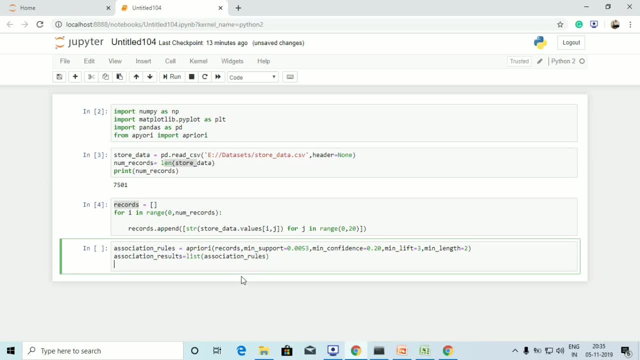 줘. Let's get the packet. Here we go. We have created the list, No, as we have Bill the model and convert the data into list. Now let's go ahead and view the start length again of the updated file, which is print of length and association. 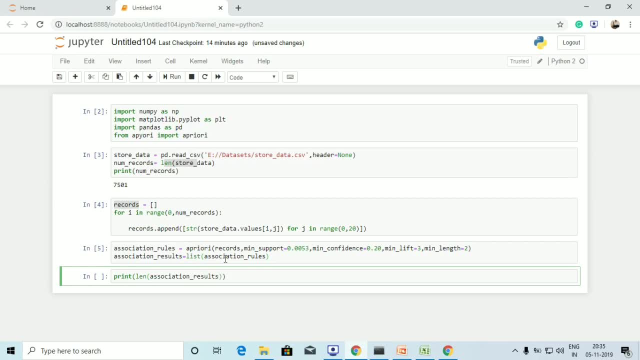 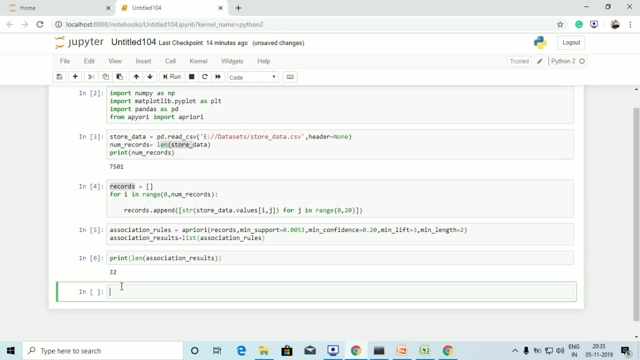 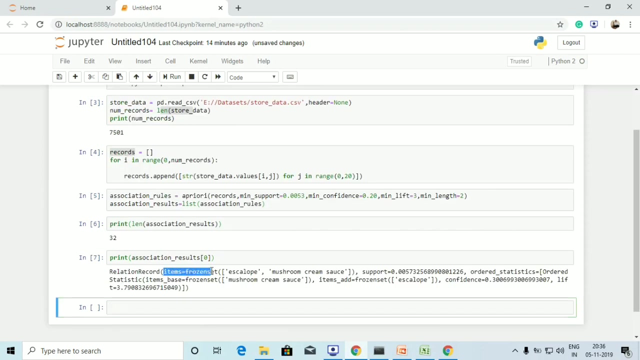 underscore results and view the exact result, what we are getting. here we go. we have the length that is 32. now let's see the first data of the association results, which is association underscore results of zero. let's go ahead and see this. here we go. as you can see, we are getting the items which is chosen. set of escale. 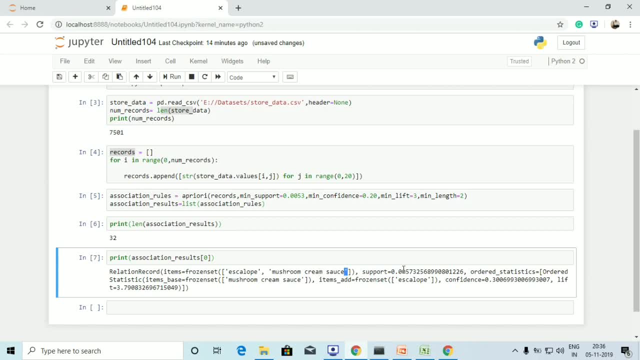 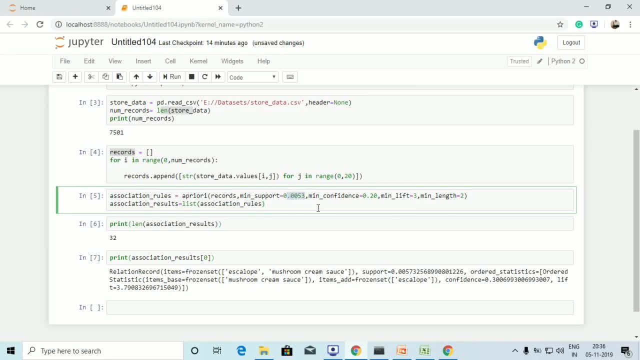 0.0057, as we have provided the minimum support value for it as 0.0053.. So it's coming beyond that. So next, we have confidence for confidence, the minimum confidence we have provided as 0.20.. So, as you can see, it's coming bigger than that which is 0.30. similarly for lift. 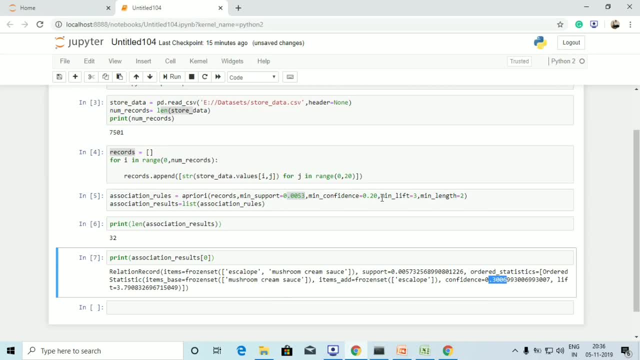 as well, which is 3.79.. The value file, as we have found it for lift as 3.. So this is how we get to know the length of the file. Now let's go ahead and try to display the results in a separate column for confidence support For doing that. I'm again going to. 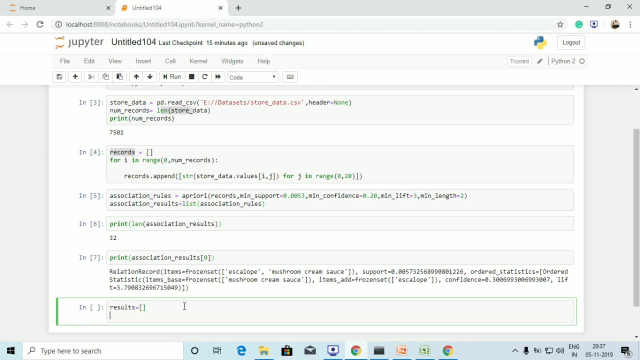 like create one more variable and name it as result. If you create just one more variable, I will name it as result. So let's go ahead results and keep it in blank, and I'm going to use follow and provide a variable called item in association underscore results. So for item in association underscore results, 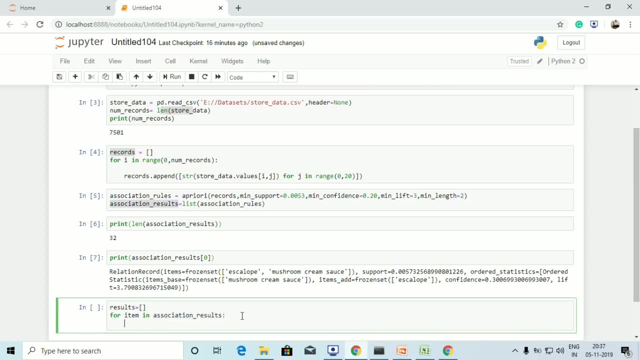 which is referring to this, and inside that I'm going to create a variable called pair, in which I'm going to store the first value of the item, which is: for item equals to item of zero. then I'm going to use the variable item and open the bracket which is: and give: 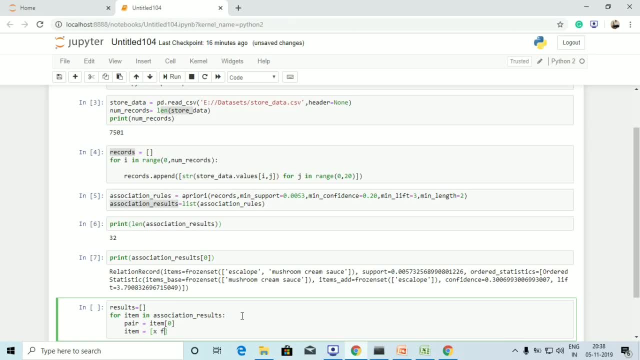 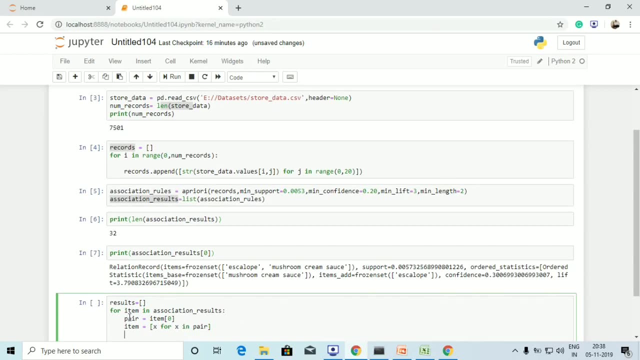 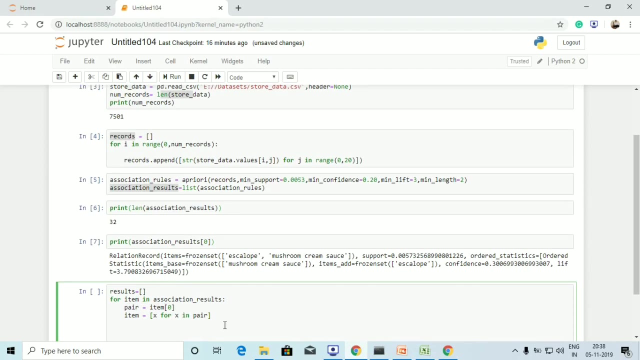 a variable called x and one more follow, which is x for x in pair, which is this variable for adding this item of zero. So here we go. Now let's try to put four to five values, which is by creating a variable called value of zero equals to using a string and inside. 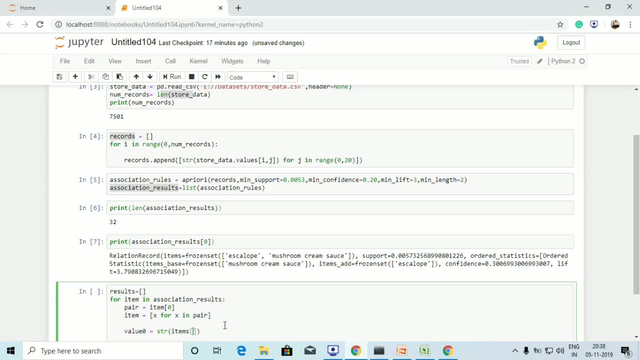 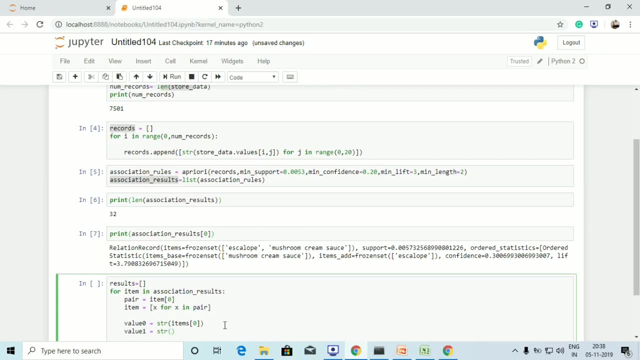 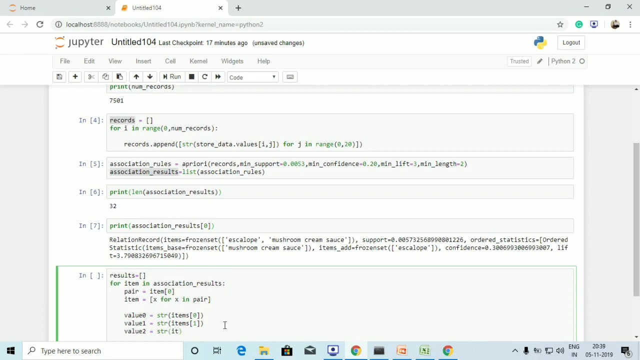 the bracket. Let's say, one more variable for items of zero. Now, similarly, for value one, I'm going to provide string of string of items of one. two things are created. now for value two, Let's go ahead and create one more, which is item. here we are going to provide the item, not items. Okay, so, with item and ending this, 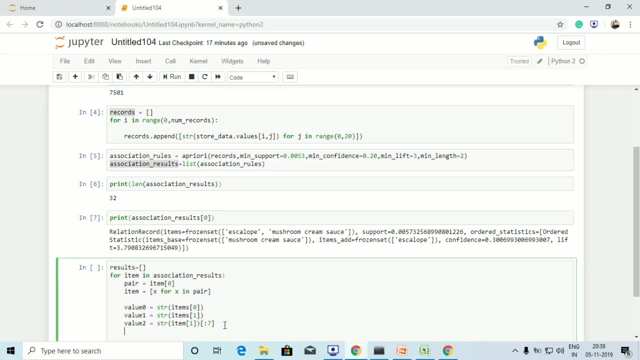 with seven, make sure that it ends within seven and for value three. similarly we do that by acquiring again item. here we give to the second and zero to 202, which means second item, that is item of two, zero and two and end is seven. So we have created value of zero, one, two and three. Let's 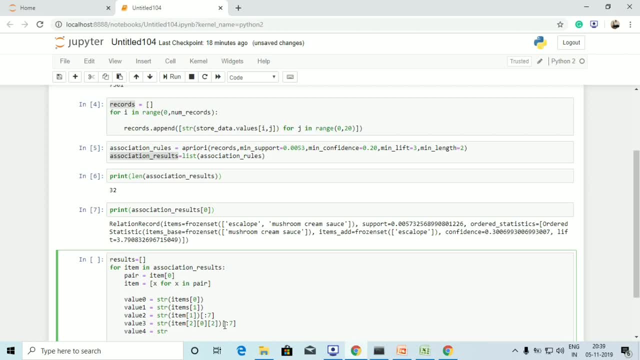 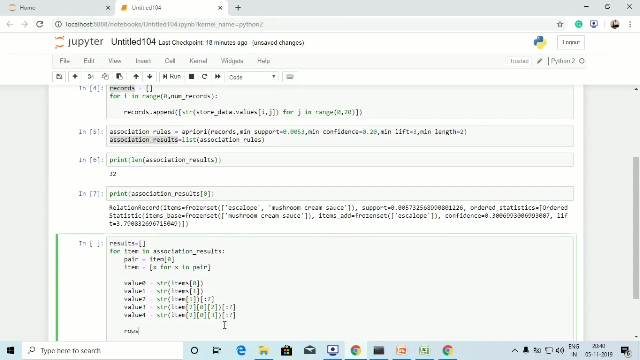 go ahead and create again. We are going to provide your four, which is string, again with item Oh, two, zero and three and end this by within seven. So here we go. we have created the value of zero, one, two, three and four. Now let's store this in a variable which I have defined right now, and rows and: 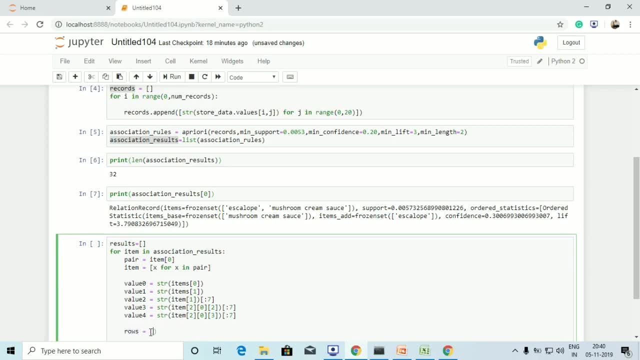 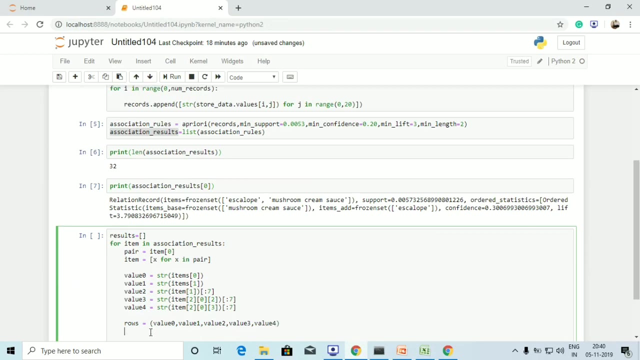 and store this in rows as like: value of 0, comma. value of 1, comma. value of 2, comma, value of 3, comma, value of 4.. So here we go. we have created the rows, that is, variable rows, and set up the values. 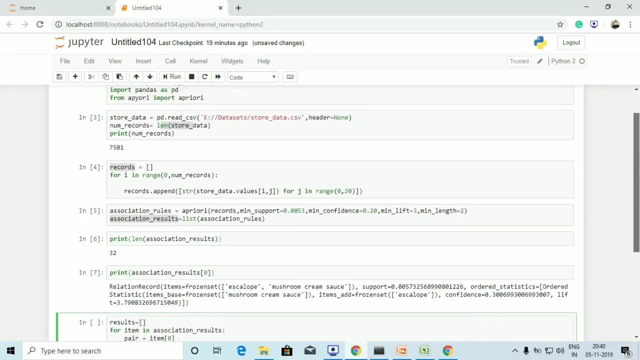 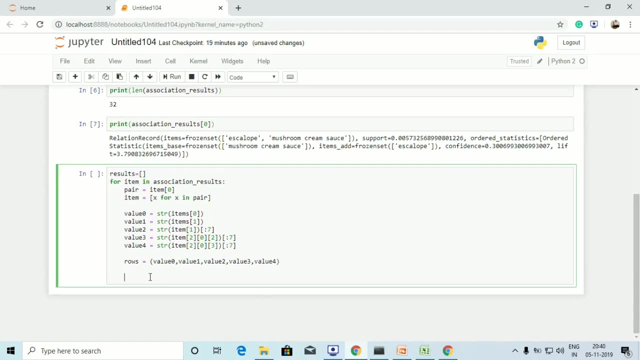 Now let's try to append again, just like what we did here, in records. It is record sort append to make sure all the values are coming under 1.. So for that I'm going to use again which is resultsappend, again which is append over here. 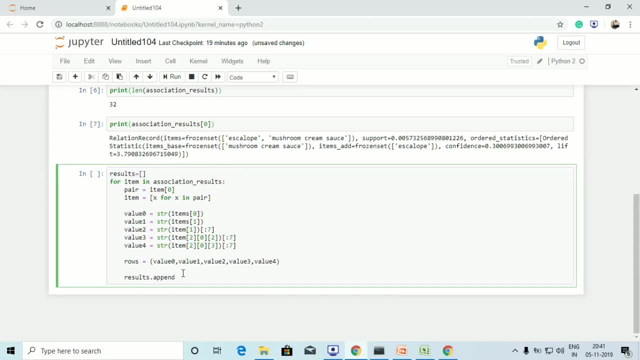 So we are going to use resultsappend and, inside the right parentheses, I'm going to pause the rows which have created variable in which all the values are stored. Now, what is required? We require a label as a header to for a header. 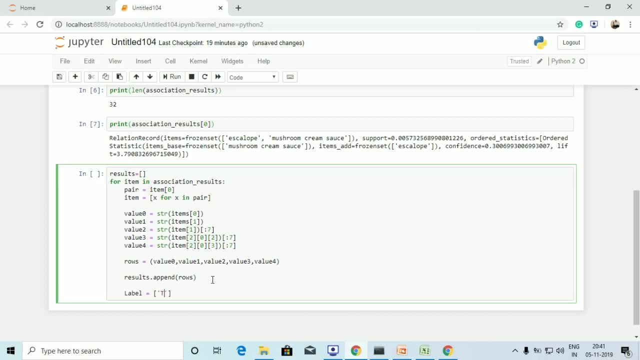 So we require a label which is, let's say, title1, comma, title2, comma. then what will be required? We require support and we require confidence, Followed by we require left. Here we go: We have created a label. Now we need to put this into a data frame. 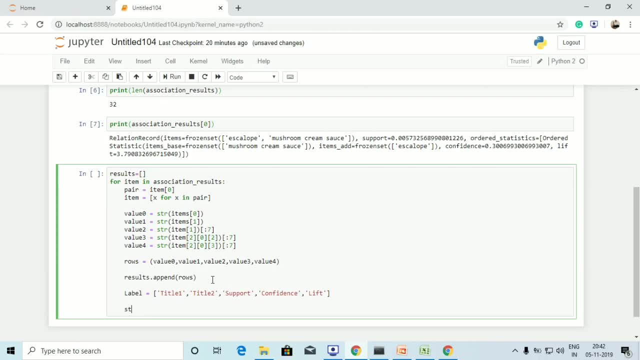 by using PD. It is fantastic. for that I'm going to create a variable called store suggestion, as we are going to suggest right. So, for random example, I have you then store suggestion and inside that I'm going to provide pandas. It is pddataFrame. 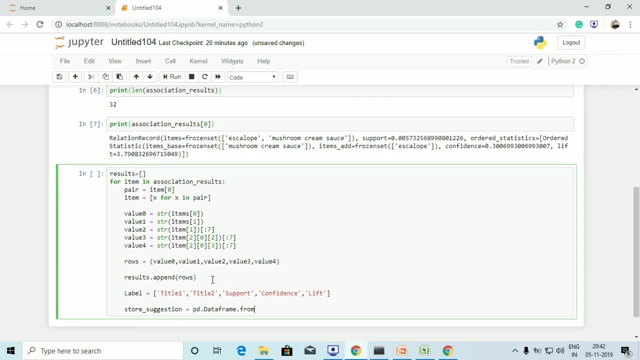 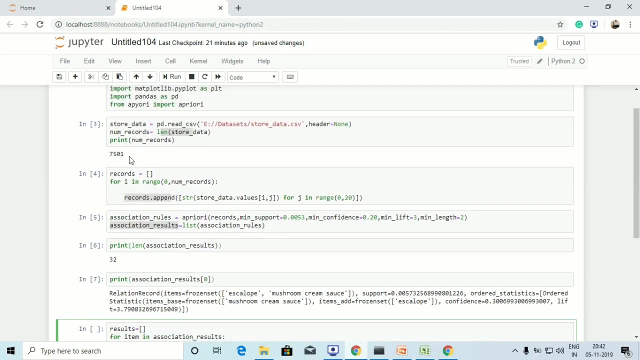 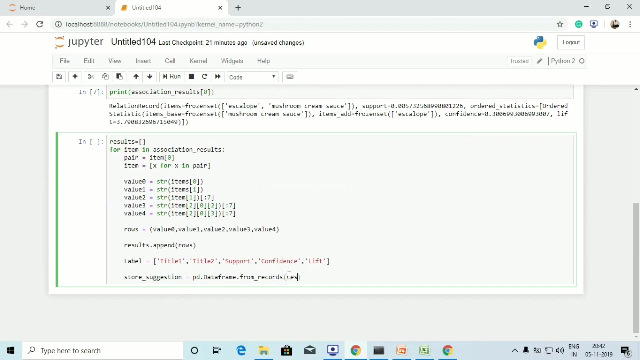 dot from underscore records, which is from underscore records, which is this: And inside the brackets, I'm going to pass on results in which our values have been stored, which is this: Along with that, I'm going to make sure my columns. 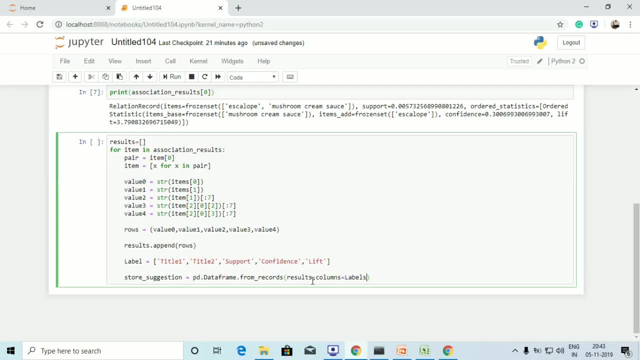 are in labels, which is one column for title, one column for title2, the support, confidence, and leave separate columns, which is column equals to labels. So we have ended with the coding part. Let's now go ahead and run the program. 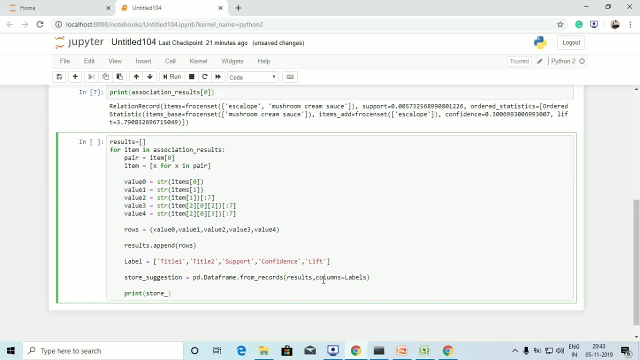 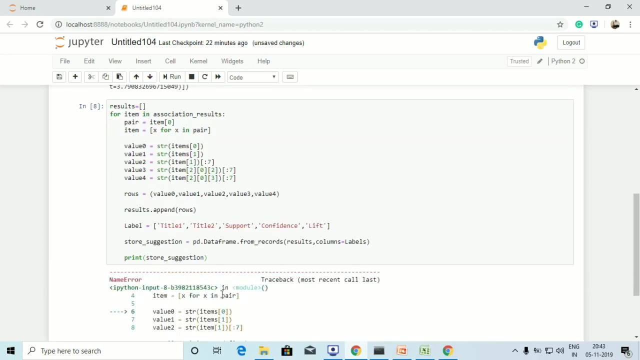 and see what we are getting in, which is print store underscore suggestion which refers to this. Here we go. We have done with the code. Let's now go ahead and run the program. What we have is an error. Name items is not defined. 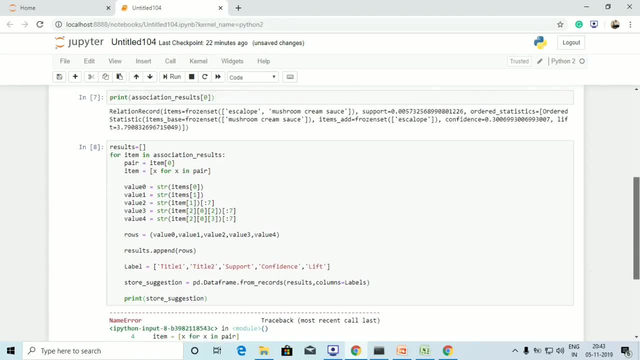 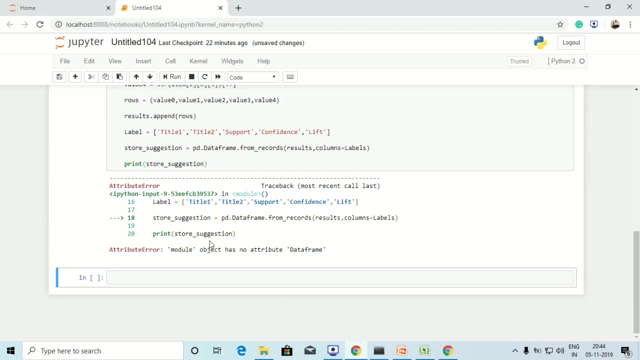 Okay, Here we go. Oops, I need to provide. Actually, I have missed an S variable. Okay, So items. Okay, Let's go ahead and I can run the program. One more error, which is label title1.2.. 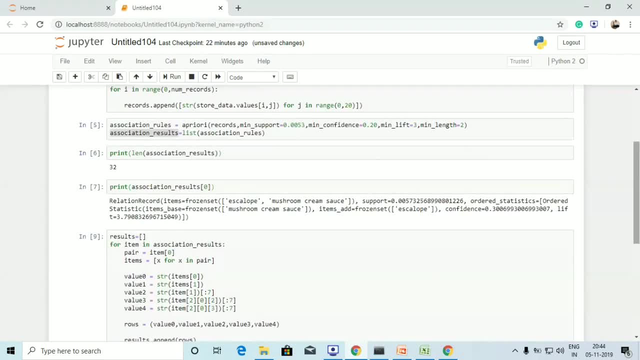 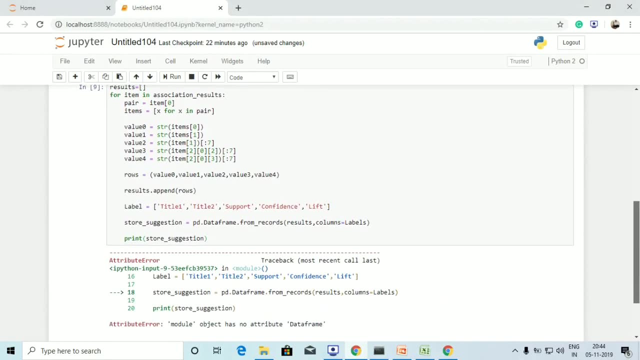 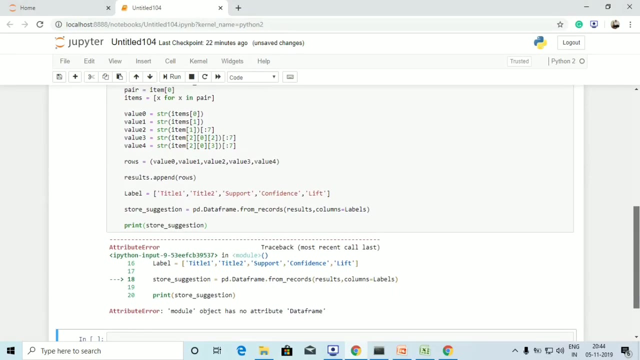 Label, title1,, title2, support, confidence and list, which is store underscore suggestion: pddataframe: confirm underscore records. We have missed something. Let's check out. Okay, We have missed the label. Let's now go ahead and run the program. 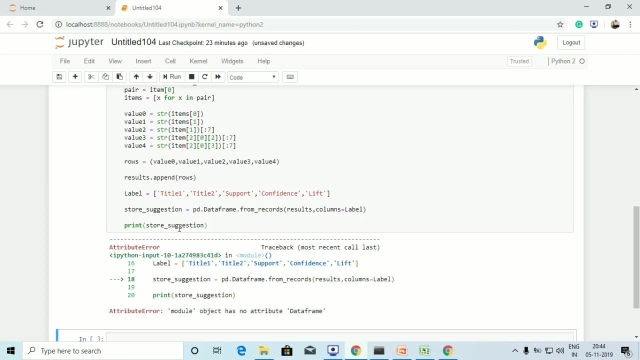 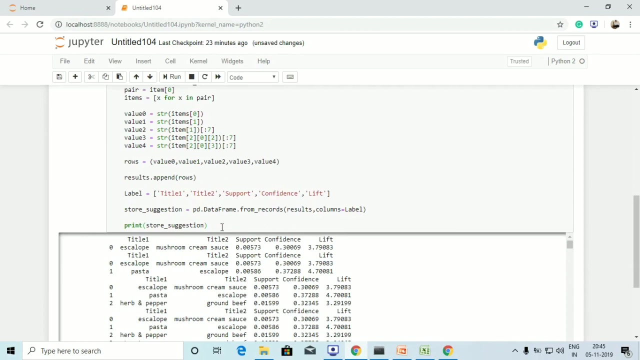 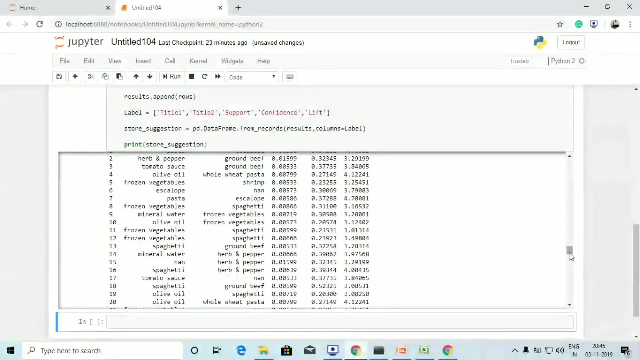 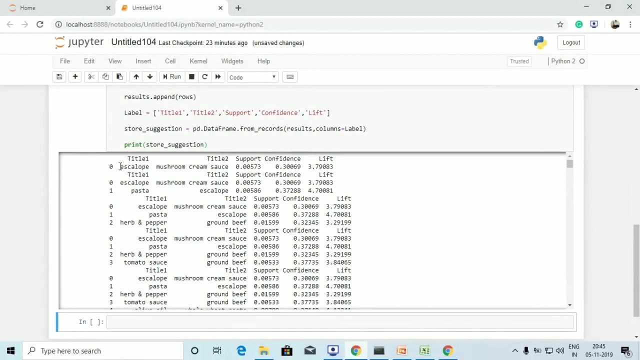 Again. print store underscore suggestion. Everything is correct. What is the problem? Here we go As expected. as you can see, we are getting the output in separate columns. Let's say, the title1, first one is a scallop and the title2 is mushrooms cream sauce.